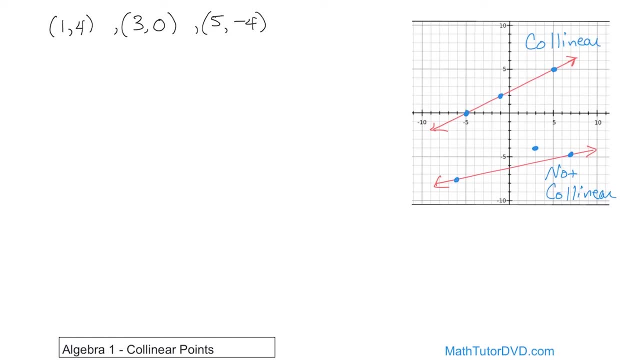 that you figure it out. you could plot it, of course, and draw a line through them, but the way you mathematically figure it out is you say: all right, look at these three points here. If you were to calculate the slope between these two points, what would you get? Well, let's just pretend for a second. you got a. 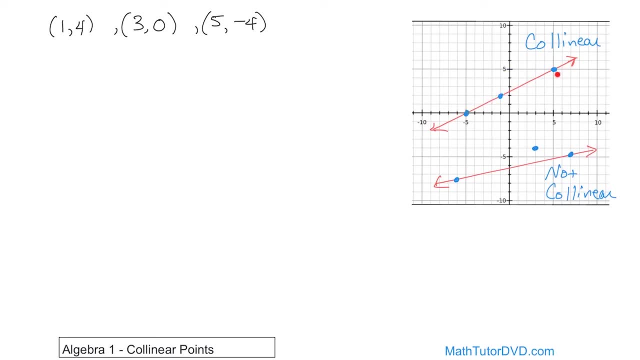 slope of one-half right. and then let's say you were to calculate the slope between these two points. Well it, since they're all along the same line, the slope between these two points should be exactly the same as the slope between these two points. or if you? 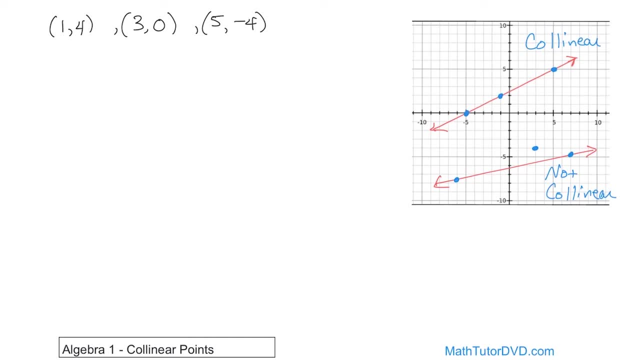 calculate the slope between this one and this one, you should also get exactly the same thing. So when points are collinear, the slope that you calculate between any of those points is always going to be the same, because they're all on the same line right Now. compare it with this, If I can calculate the slope between these: 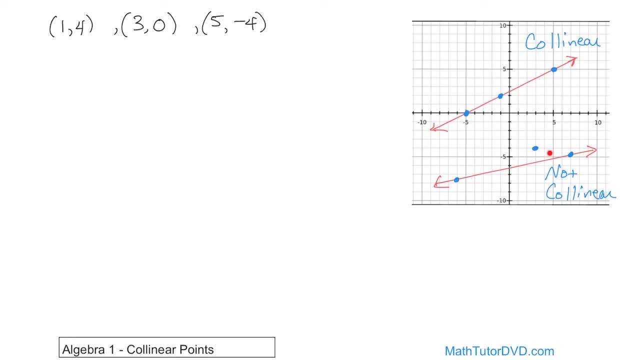 two points right here I'm going to get a different slope than if I calculate the slope between these two points. So the test for collinearity is basically: take the three points here, Let's calculate the slope between these two points and we'll get a number, And then we'll calculate the slope between these two points. 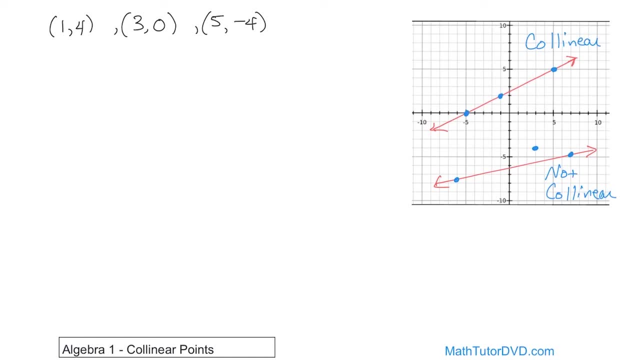 and we'll get a number. If we get the same number, then we know they're collinear, And if we don't, then we know that they're not collinear. So that's what we're going to do. So the way you're. 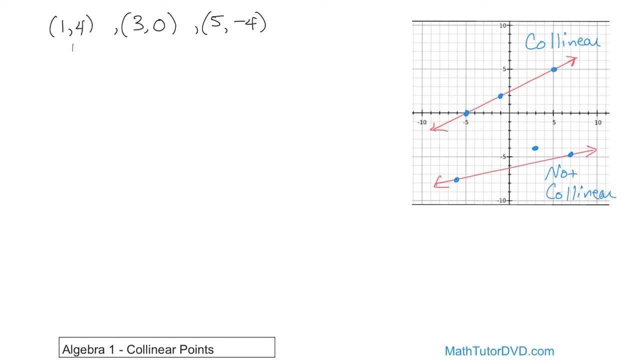 going to handle this. to keep it straight, we'll call this: we're going to calculate the slope between these two, We'll call it M1, and we'll calculate the slope here between those two points, We'll call it M2.. So let's go ahead and calculate M1 and M2.. So M1 is y minus, y minus over x minus. 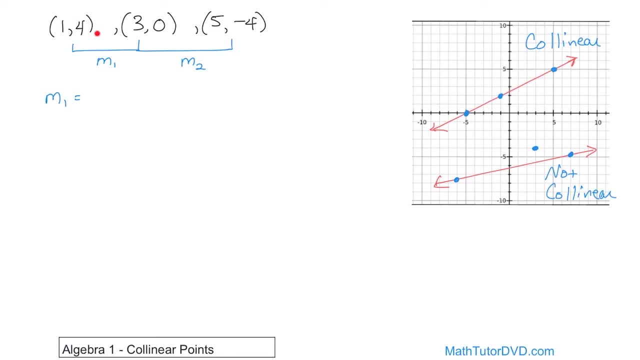 x1.. So the difference in the y is the difference of the x's, And we go the same direction: 4 minus 0 here, on the top, 4 minus 0. And on the bottom we have to go the same way: 1 minus 3.. So what we? 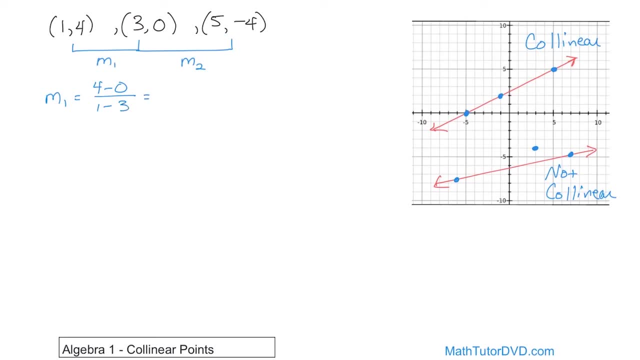 get is: let's do it like this: We'll do 4 minus 0,, so 4.. On the bottom, we get negative 2. And so you divide those, you get negative 2. So the slope for M1 is negative 2.. 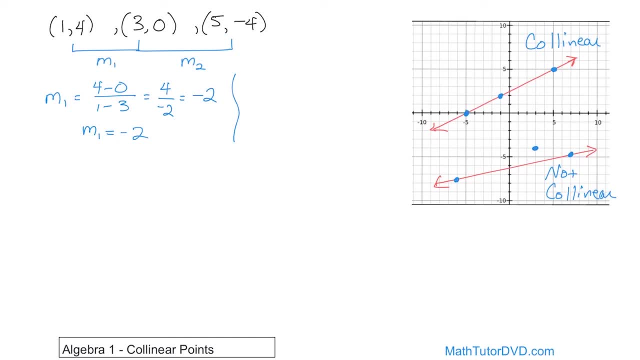 There you go. Now let's calculate the slope M2, which is the slope between these two points right here. So we'll do the same thing. It's the difference of the y's on top. We'll go this direction: 0 minus negative 4, 0 minus negative 4 on the top. And since we went that way, we have 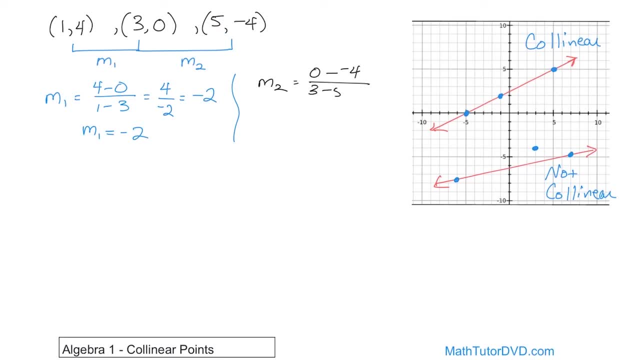 to do 3 minus 5, 3 minus 5.. So what we'll do here is we'll add the opposite And on the top we just get positive 4.. On the bottom, we get negative, 2. So the slope M2,. 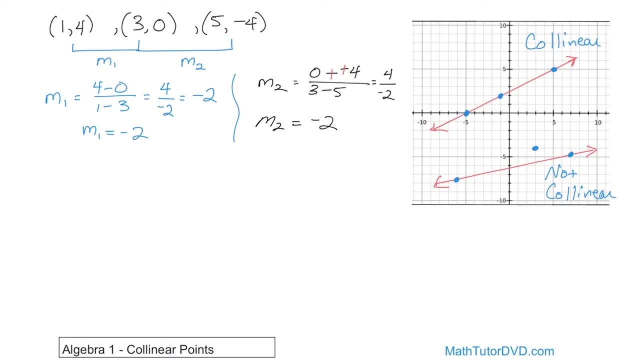 is equal to you divide those, you get negative 2. So these are the same slope, So these are collinear, All right, so that's what you would circle, You would calculate both slopes and you would say that they were collinear If you were to calculate the slope between these two points. 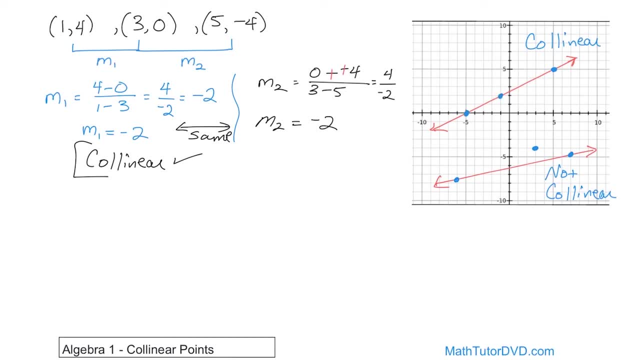 you would find the same thing, Because if this slope is equal to this one, and this slope is equal to this one, then of course the end points are always going to have the same slope too there, So you don't have to calculate that third one. 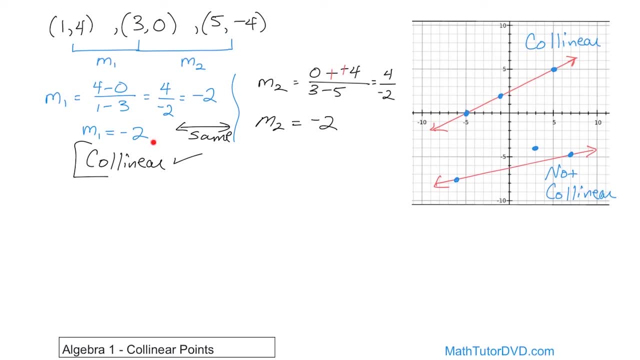 Let's go between and calculate everything in between. If you get the same number, then you're going to be saying that these are collinear points. All right, let's go ahead and take another example. Let's give me- I'll give you- three additional points. Let's say: negative 5, 9,. negative 1, 1,. 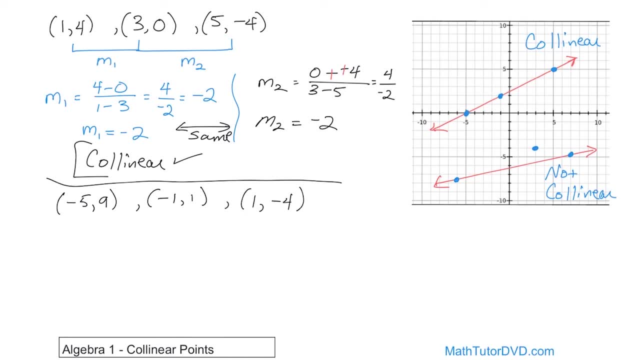 and 1, negative 4.. And we're going to calculate the slope between them. Now we're going to call this one M1, and we'll call this one M2, just to keep it clear. Let's calculate M1 right over here. So let's go 9 minus 1 on the top, the difference in the y values. 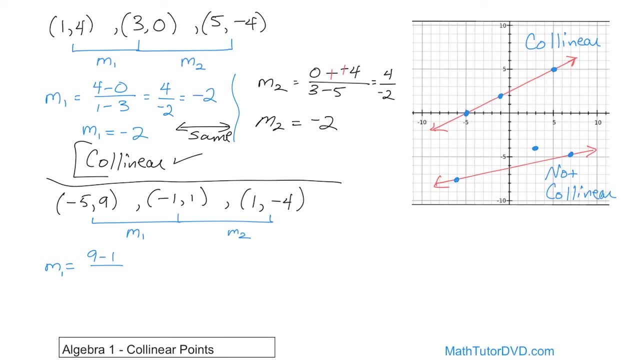 When we go that direction, then we also have to have the negative 5 minus negative 1, negative 5 minus negative 1.. On the top, 9 minus 1 is 8.. On the bottom, we have to add the opposite. So what? 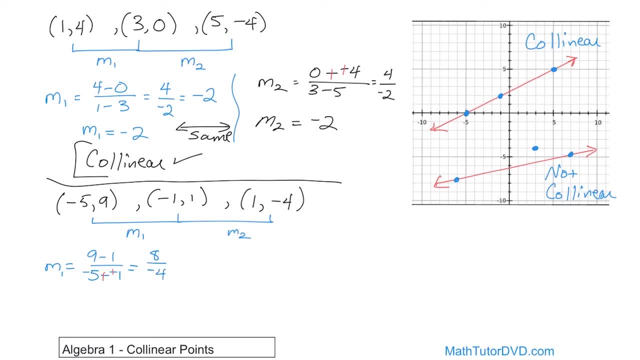 we have is negative 5 plus 1, which is negative 4, which means we get negative 2 for an answer here. So M1 is negative 2, same as previous problem. That's just a coincidence, though, And now let's go calculate M2 between these two points. 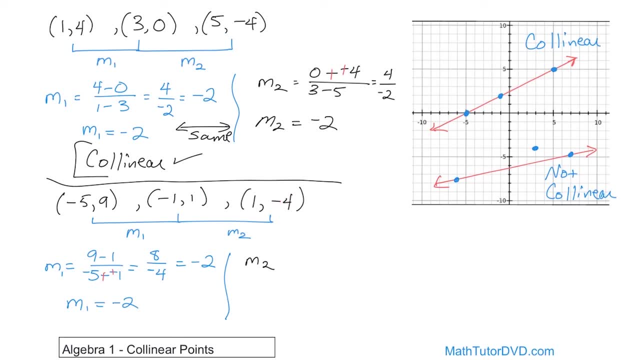 So what we'll do is we'll say: for this one we'll go 1 minus the negative 4, 1 minus negative 4. on the top And on the bottom it will be negative 1 minus 1, negative 1 minus 1.. So what we will have is adding the opposite, just like that on the top.